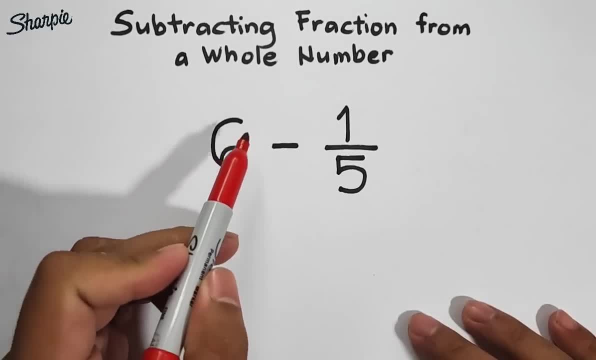 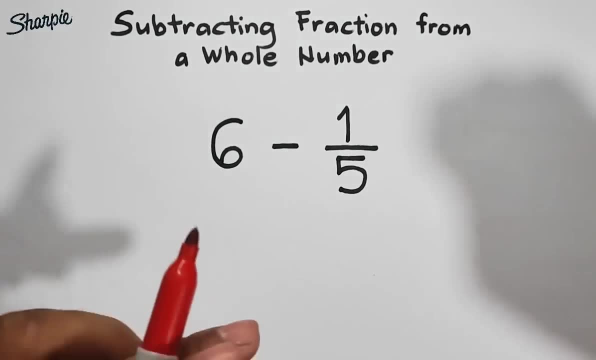 given example: your 6 is the whole number and 1 over 5 is your fraction. So the question here: how are we going to subtract 1 over 5 from this whole number? So let's try solving this. So I will. 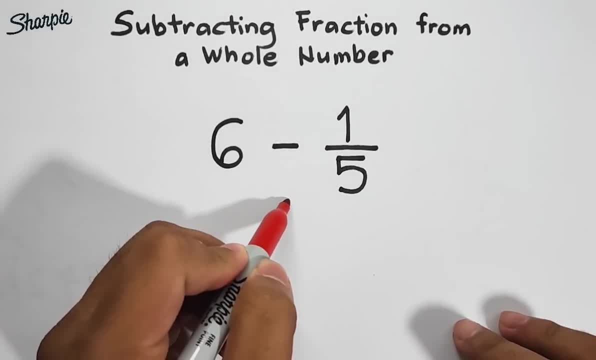 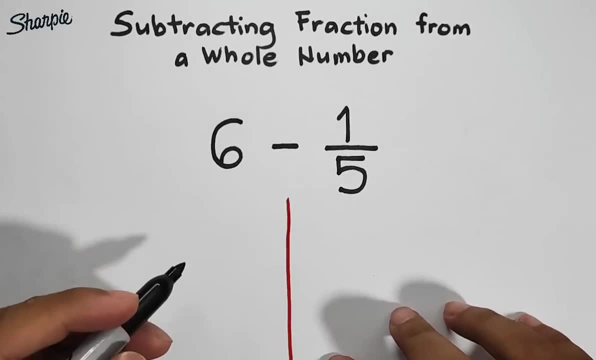 show you two different methods on how to subtract this. Okay, so let's use separation. and in this case, guys, let's start with method number 1.. So let's use method number 1.. Now, here's the case, guys. Let's start with method number 1.. So let's use method number 1.. Now, here's the case, guys. 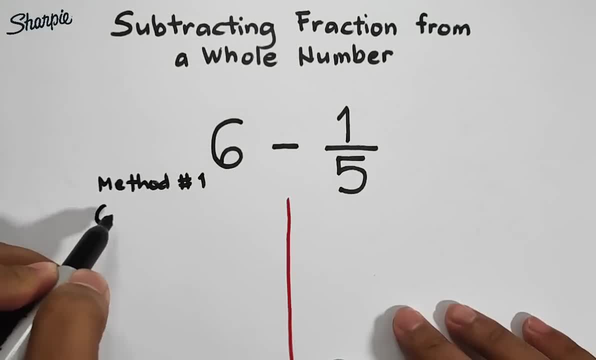 We have 6 minus 1 over 5.. This whole number has its invisible denominator, which is 1, so we can rewrite it as 6 over 1.. So, as you can see, our new fractions are 6 over 1 minus 1 over. 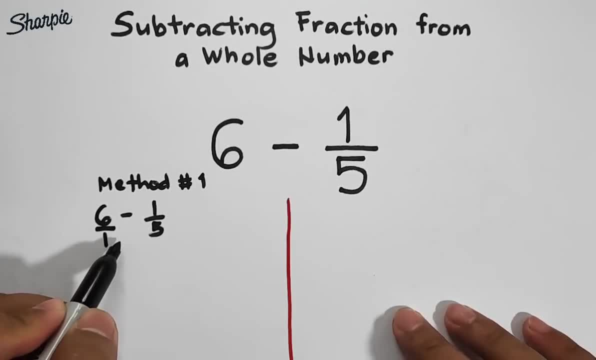 5, wherein we need to get the LCD of these two denominators, which is equal to 5.. So next process is that we will subtract this or divide this by 1 and then multiply by 6.. So 5 divided by 1 is 5 times 6, that is equal to 30.. Minus 5 divided by 5, that is 1, times 1.. That is. 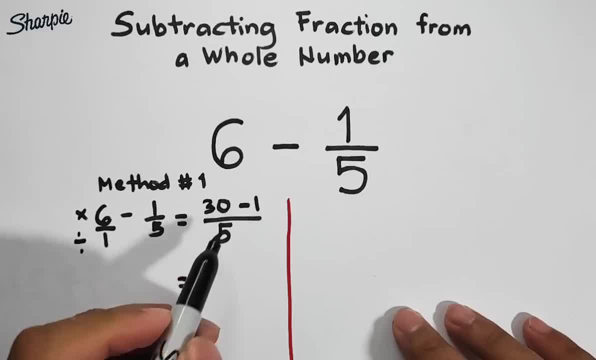 also equal to 1.. so what we have here is 30 minus 1. That is, 29 minus 4.. So we can substitute the 29 over 5.. So we can consider this as our final answer, But in case that your teacher asks you for another answer like convert this into mixed number, 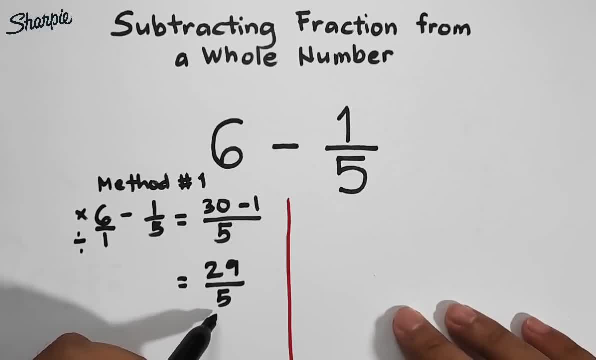 the value or the equivalent mixed number of this is this: 29 divided by 5,, ilang 5, or how many 5s do we have in 29?? We have 5.. So that will be the whole number of your mixed number. 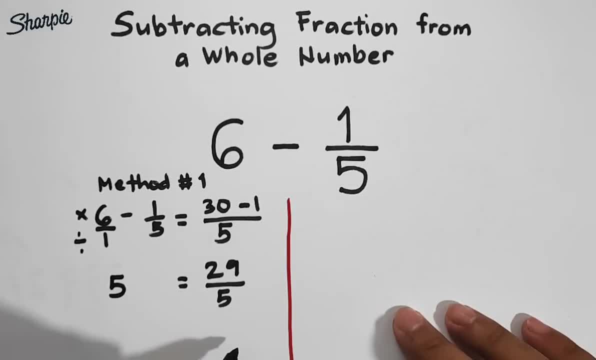 Next. so by dividing 29 by 5, we have 5, and then the remainder is 4.. So that is the new numerator over copy your original denominator, which is 5,. so that will give you 5 and 4 over 5, and that is also equal to 29 over 5.. 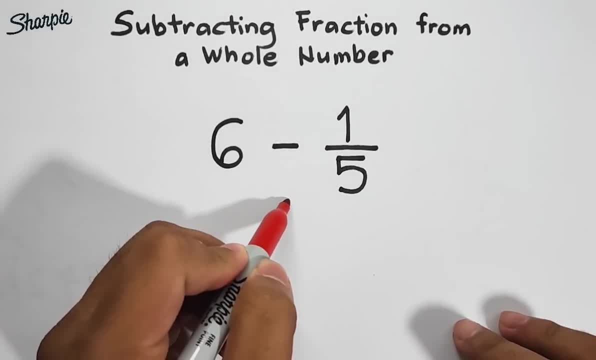 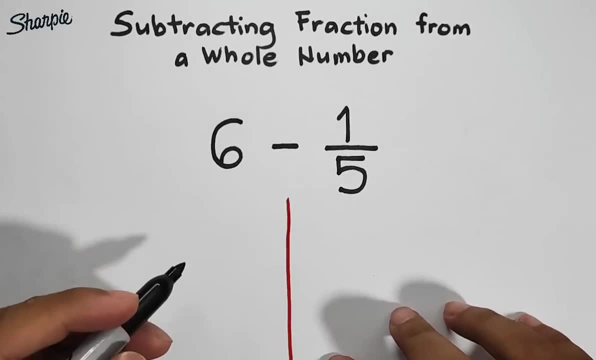 show you two different methods on how to subtract this. Okay, so let's use separation. and in this case, guys, let's start with method number 1.. So let's use method number 1.. Now, here's the case, guys. Let's start with method number 1.. So let's use method number 1.. Now, here's the case, guys. 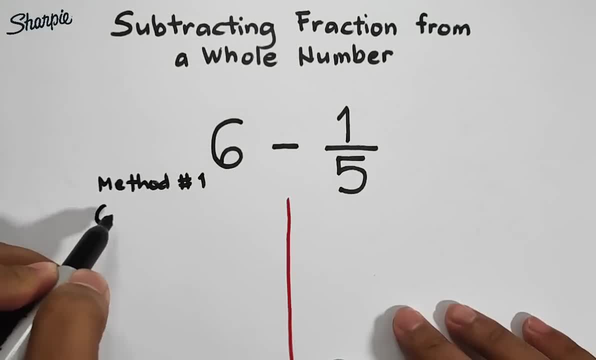 We have 6 minus 1 over 5.. This whole number has its invisible denominator, which is 1, so we can rewrite it as 6 over 1.. So, as you can see, our new fractions are 6 over 1 minus 1 over. 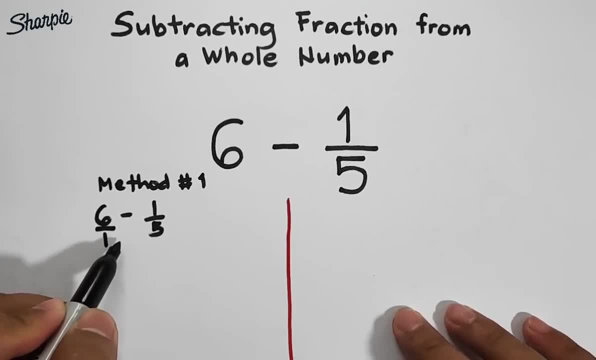 5, wherein we need to get the LCD of these two denominators, which is equal to 5.. So next process is that we will subtract this or divide this by 1 and then multiply it by 6.. So 5 divided by 1 is 5 times 6, that is equal to 30 minus 5 divided by 5, that is 1 times 1, that is. 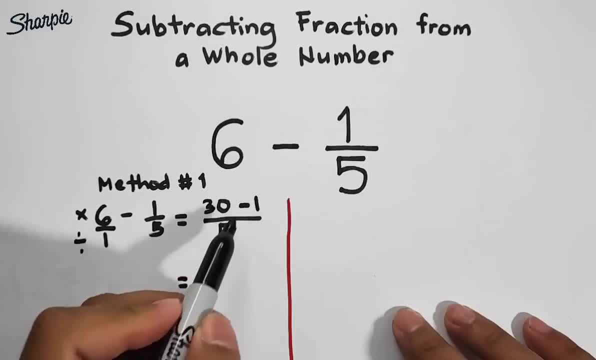 also equal to 1.. So what we have here is 30 minus 1, that is, 29 plus 1 plus 1.. So here we over 5, so we can consider this as our final answer. but in case that your teacher ask you for another another answer like: convert this into mixed. 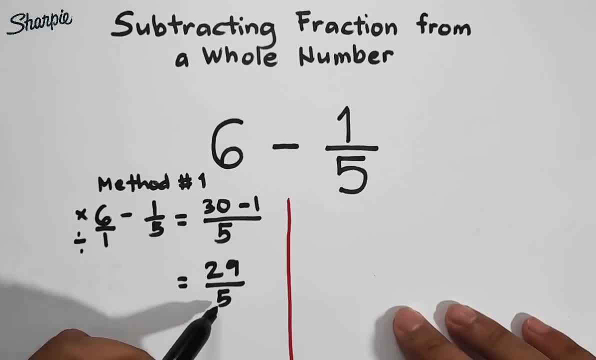 number, the value or the equivalent mixed number of this is this: 29 divided by 5, ilang 5, or how many fives do we have in 29? we have 5, so that will be the whole number of your mixed number. next, so, by dividing 29 by 5, we have 5. 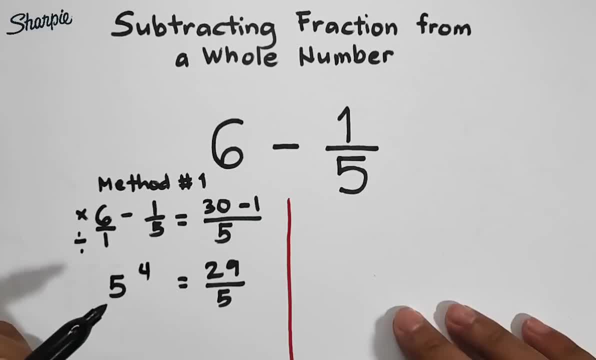 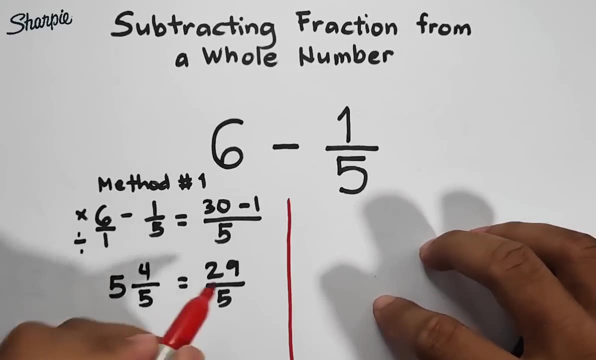 and then the remainder is 4. so that is that that is the new numerator over. copy your original denominator, which is 5, so that will give you 5 and 4 over 5, and that is also equal to 29 over 5. so we can consider this as our final answer. 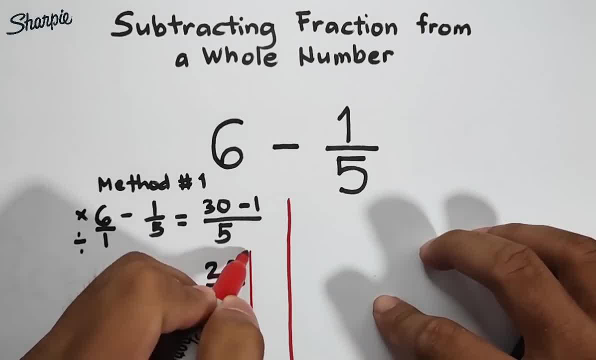 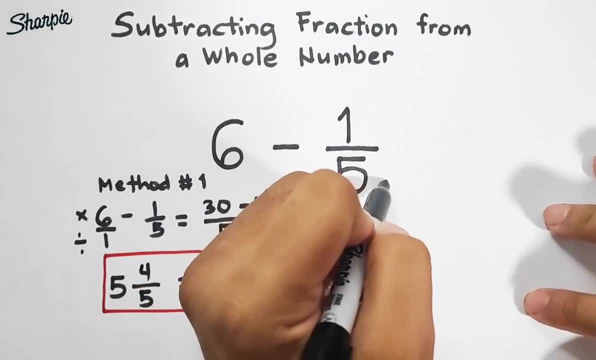 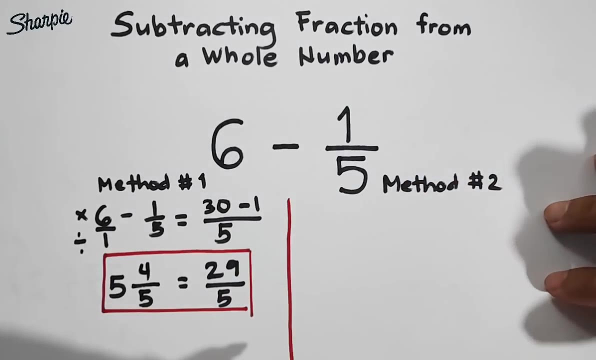 So we can consider this as our final answer. Now for the second method that we have. so let's use the second method. Let's try using method number 2.. Okay, for the method number 2, we have 6 minus 1 over 5.. 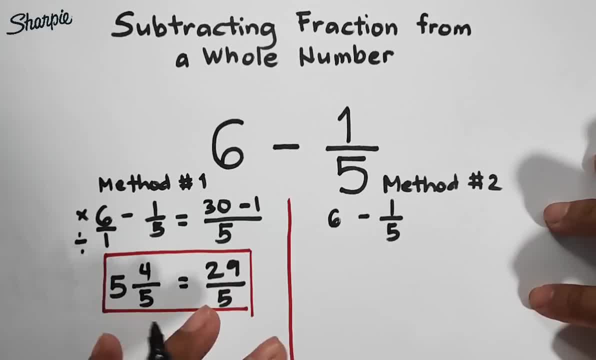 Now. so for this technique I will be doing, I will express 6 as a fraction. Okay, by the way, guys, as you can see, this is your denominator. here is 5.. To express this into a fraction, I will multiply 6 by 5, and that is 30.. 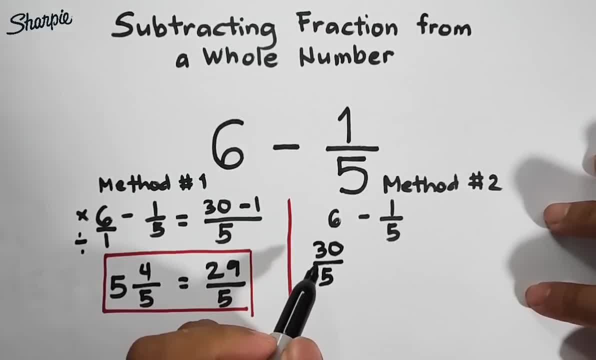 And I will copy the denominator, which is 5.. So, as you can see, when we simplify 30 over 5,, that is also equal to 6.. Again, how did I do it? I multiplied it in the denominator, which is 5 times 6,, 30, and then copy the original denominator. 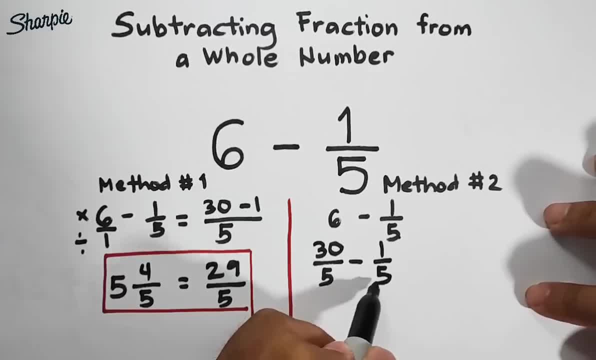 And subtract, or minus 1 over 5.. So in this case, guys, as you can see, we don't need to find the LCD or the least common denominator, because they have the same denominators. So what we need to do is to simply copy your denominator, which is 5, sorry, which is 5.. 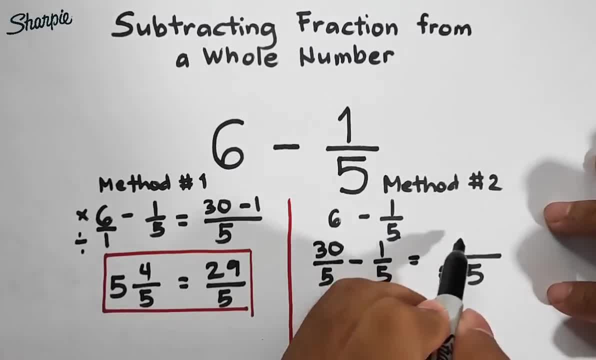 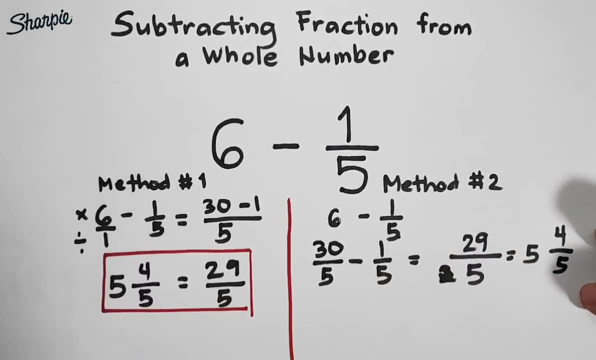 And then subtract the numerator, which is 30 minus 1.. That would give you 29.. And they will both come out the same, And still the equivalent. the equivalent mixed number is 5 and 4 over 5.. This is the answer for this problem. 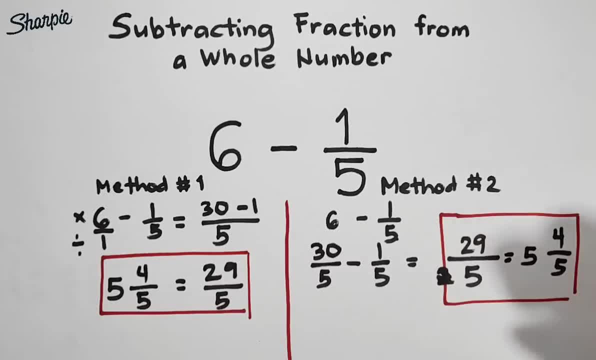 So I hope, guys, that you learned something from this video. So I will give you an assignment For our assignment. I will ask you to answer: What is 7 minus 2 over 3?? You can use either method, number 1,. 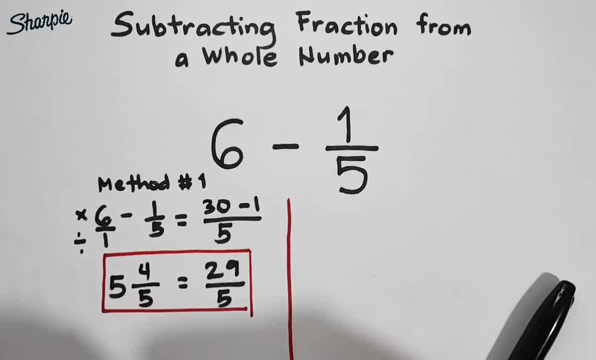 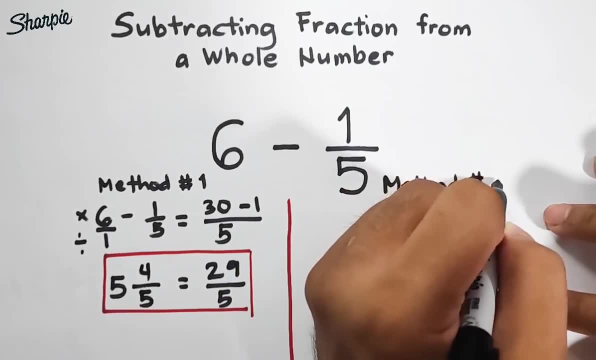 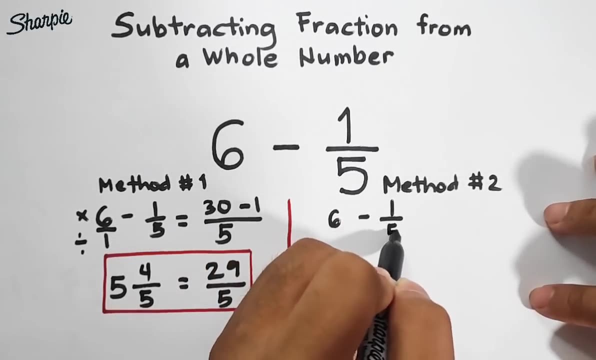 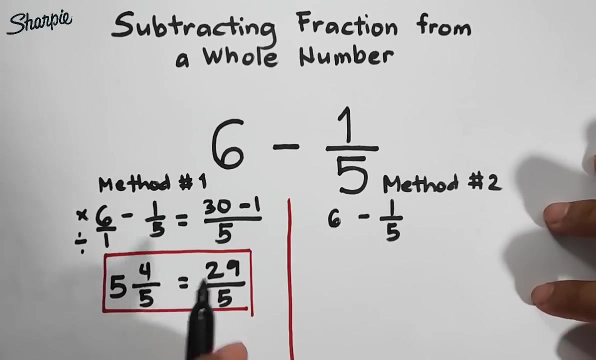 now for the second method that we have. so let's use the second method. let's try using method number 2. okay, for the method number 2, we have 6 minus 1 over 5 now. so for this technique I will be doing, I will express 6 as a fraction. 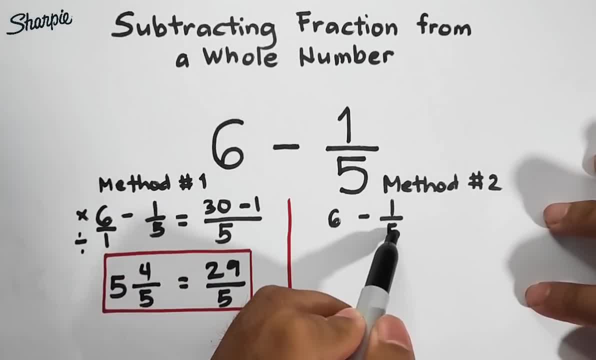 again. we guys. as you can see, this is your denominator, here's 5. to express this into a fraction, I will multiply 6 by 5 and that is 30 and I will copy the denominator, which is 5. so, as you can see, when you simplify 30 over 5, that is also. 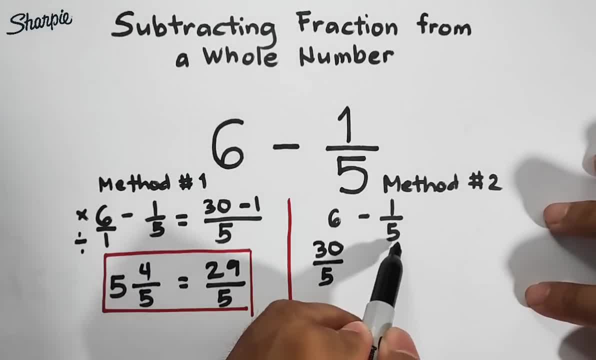 equal to 6. again, pano ko siya ginawa, multiply ko siya sa denominator, which is 5 times 6, 30, then copy it down to the denominator, then subtract or subtract, or subtract minus 1 over 5. so in this case, guys, as you can see, we don't need to find the 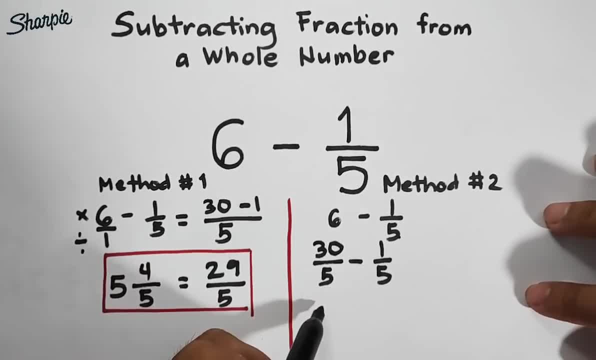 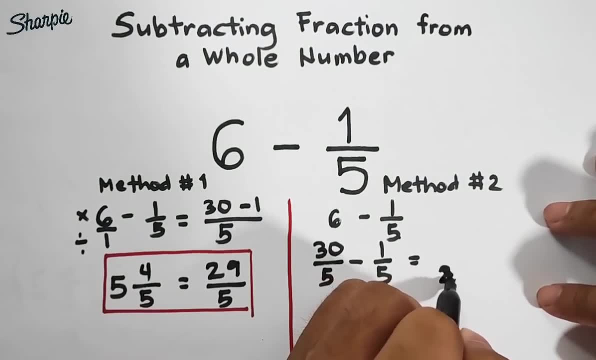 LCD or the least common denominator, because they have the same denominators. so what we need to do is to simply copy your denominator, which is 5- sorry, just 5- and then subtract the numerators, which is 30 minus 1. that would give you 29 and. 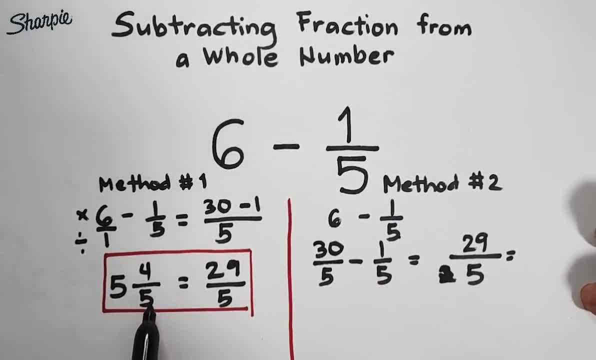 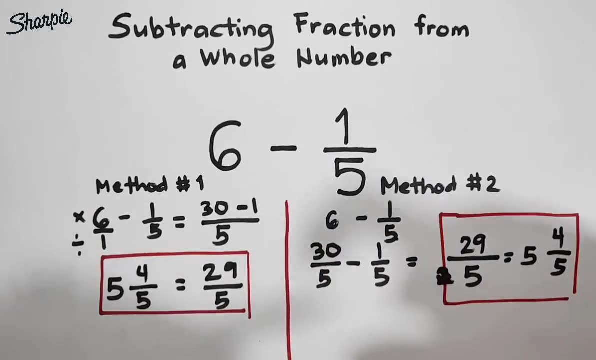 pares na silang lalabas, and still the equivalent mixed number is 5 and 4 over 5. this is the answer for this problem. so I hope, guys, that you learned something from this video. so I will give you an assignment. for our assignment, I will ask. 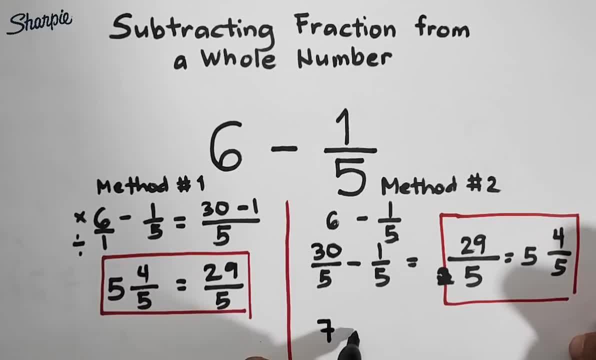 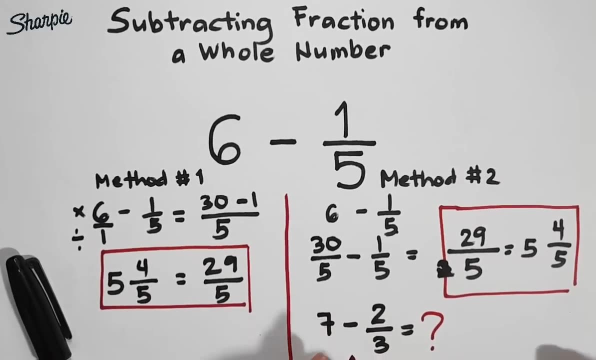 you to answer what is 7 minus 2 over 3? you can use either method number 1 or method number 2 in answering this question. so if you're new to my channel, don't forget to like and subscribe, but hit the bell button for you to be updated on our latest uploads. again, it's. 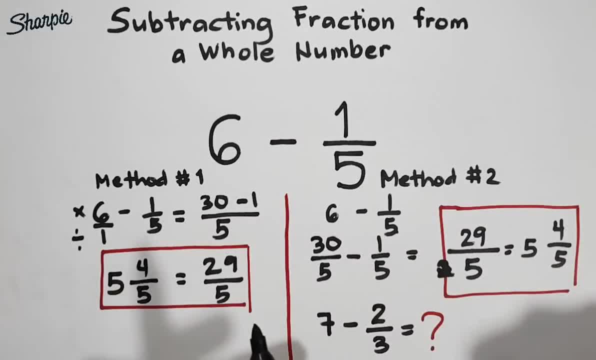 me, Teacher Gon, thank you very much. don't forget what I'm doing. bye, bye. 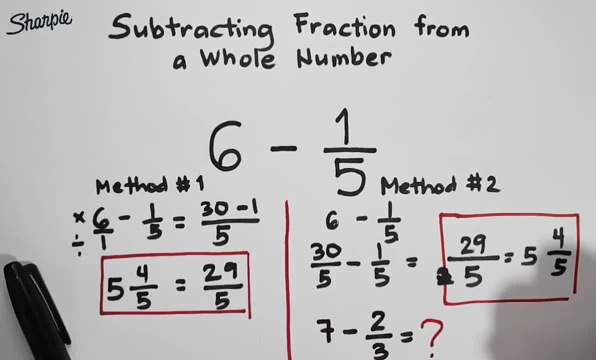 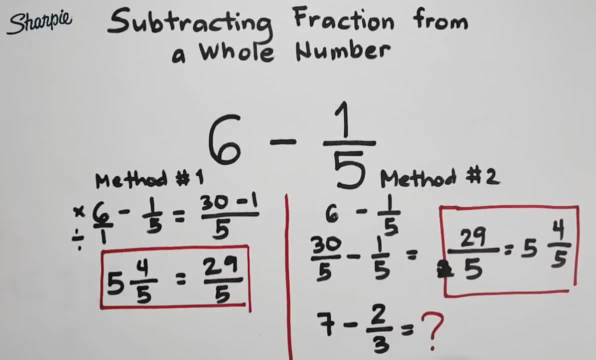 or method number 2, in answering this question. So if you're new to my channel, don't forget to like and subscribe and also hit the bell button for you to be updated on our latest uploads. Again, it's me, Teacher Gon. 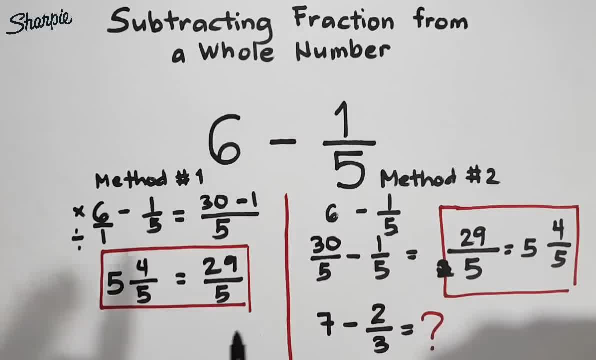 Thank you very much. Don't forget what I'm doing. Bye-bye.